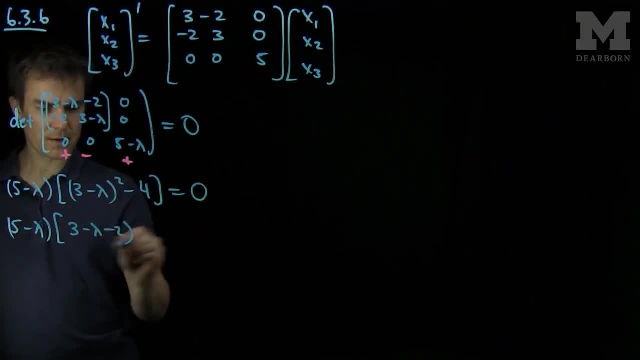 Here's the difference of two squares. So this is 3 minus lambda minus 2.. 3 minus lambda plus 2 equals 0. And from this we can find the roots. We have that lambda equals 5 from this expression over here. 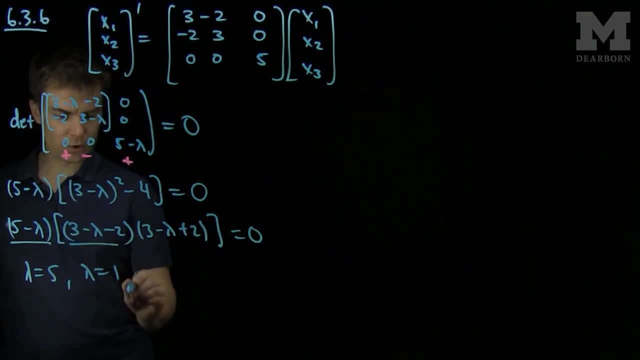 This expression over here will tell me that lambda equals equals 1 as a solution. Or if I look over here, we also get that lambda is equal to 5.. So lambda equals 5 is an eigenvalue with multiplicity 2.. 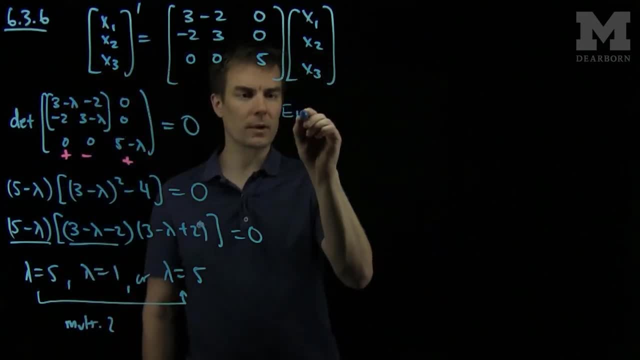 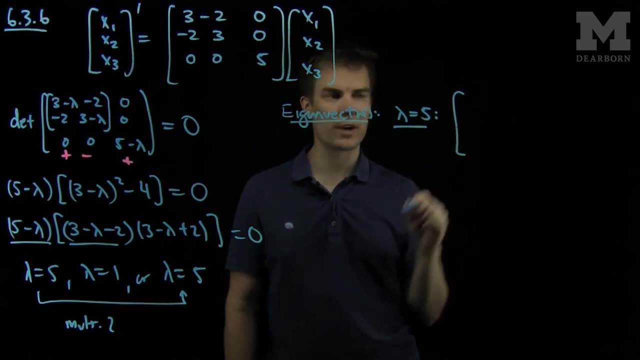 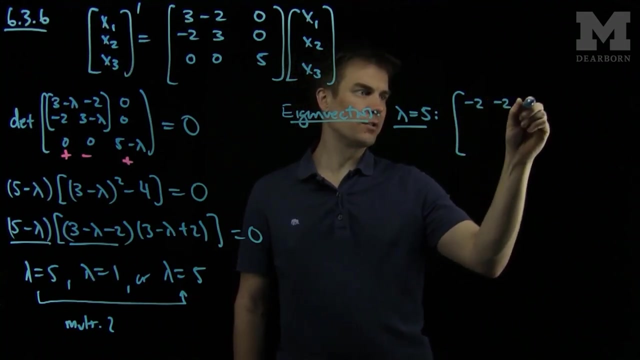 And now we need to find the eigenvectors. So the eigenvectors, The first one that corresponds to lambda, equals 5.. If we subtract 5 from the main diagonal, we'll be left with a negative 2, negative 2, 0. 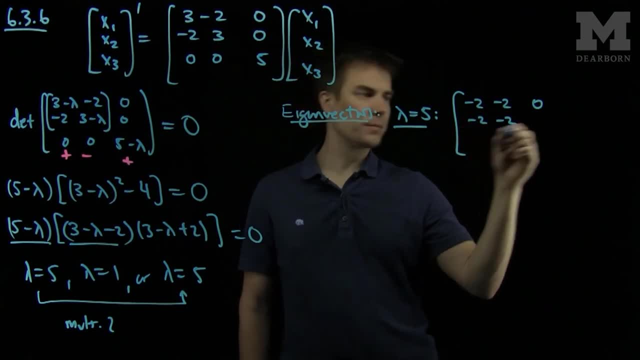 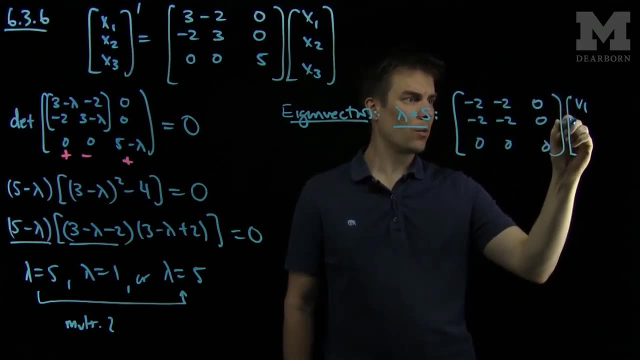 A negative 2, 0.. A negative 2, 0.. A negative 2, negative 2, 0. A 0, 0, 0 will be our matrix And I need to find V1, V2, V3. that's in the null space of this matrix. 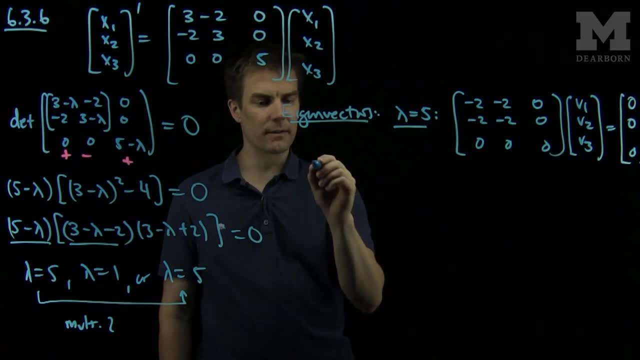 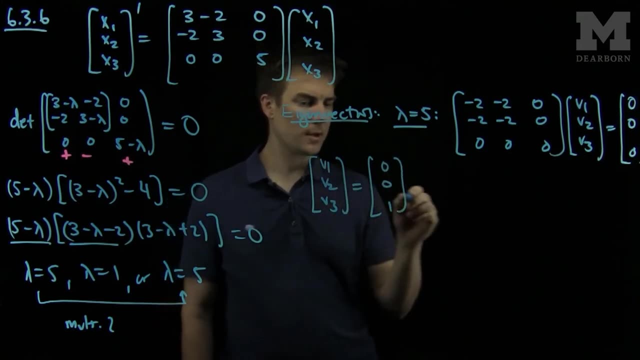 And we can see that there are two independent eigenvectors that work here: V1,, V2, V3. for choice number 1 could be 0, 0, 1.. And another choice for eigenvector V1,, V2,, V3. 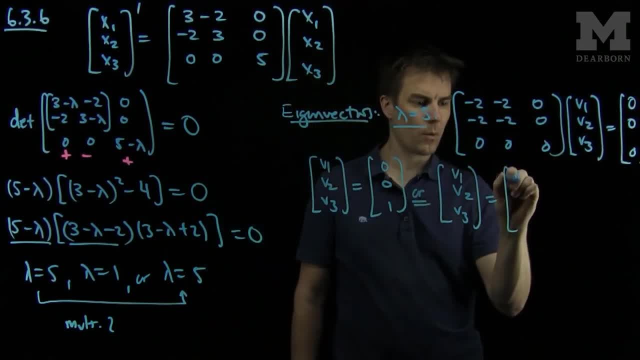 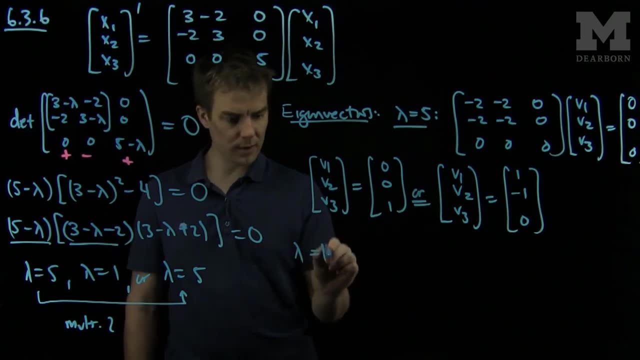 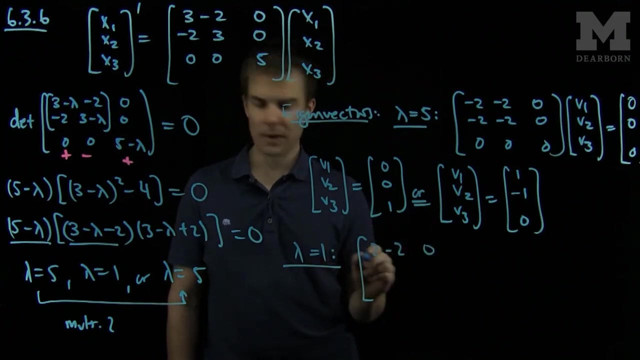 could be 1, negative, 1, 0. The eigenvector corresponding to lambda equals 1 will require us to find an element of the null space of this matrix, which will be a 2, negative, 2, 0.. Then a negative 2, 2, 0. 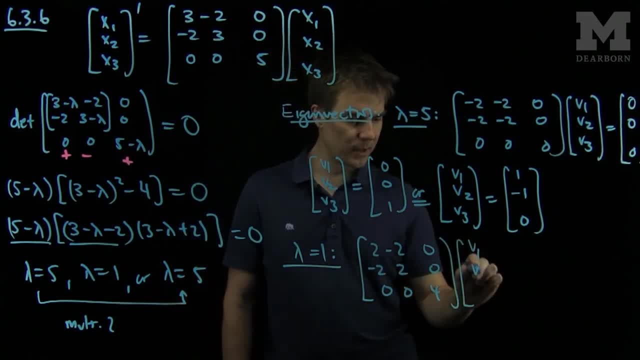 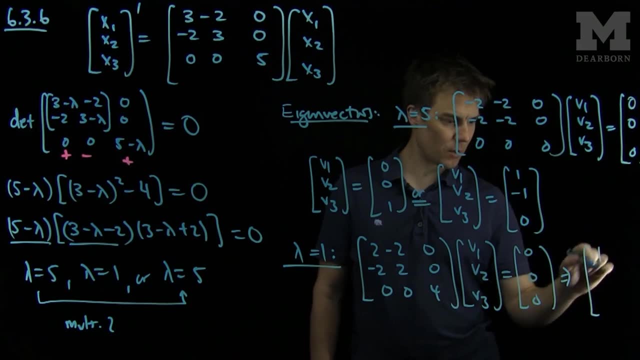 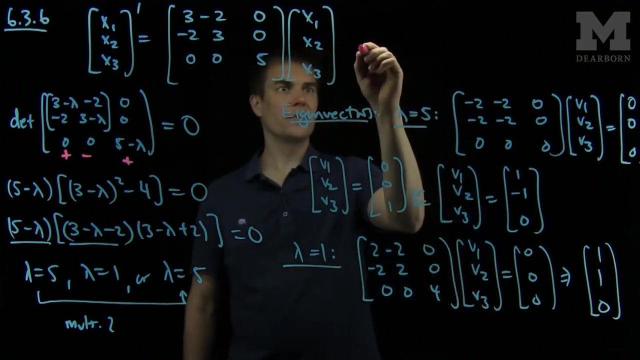 And then 0,, 0,, 4.. We can see that an element of the null space of this matrix can be found by choosing 1, 1, 0. So we can now write the solution of our problem. The solution of our problem. vector x of t. 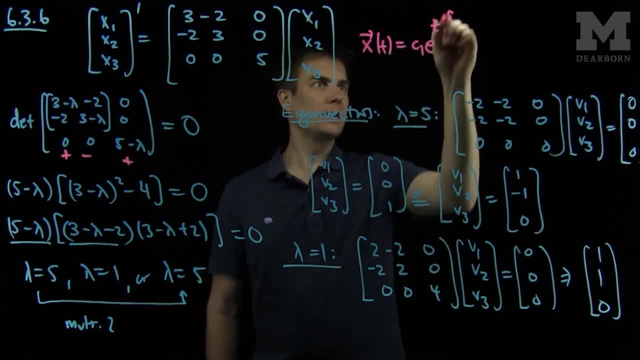 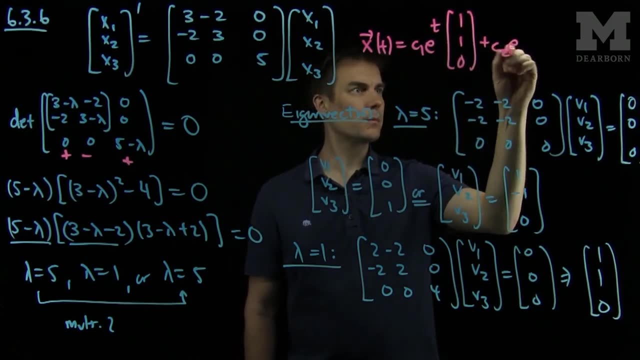 will be: C1e to the t times the eigenvector that corresponds to 1, which we found is 1, 1, 0. Plus C2e to the 5t times the vector, one of the eigenvectors that corresponds to 5..